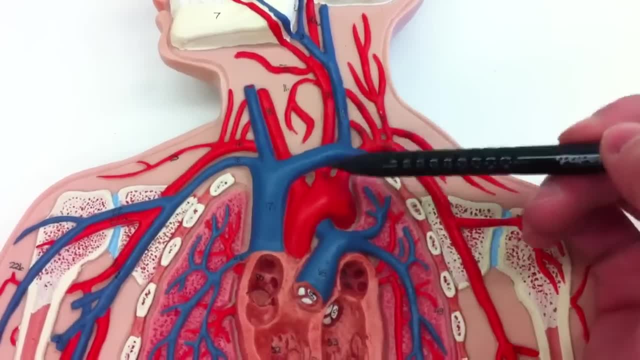 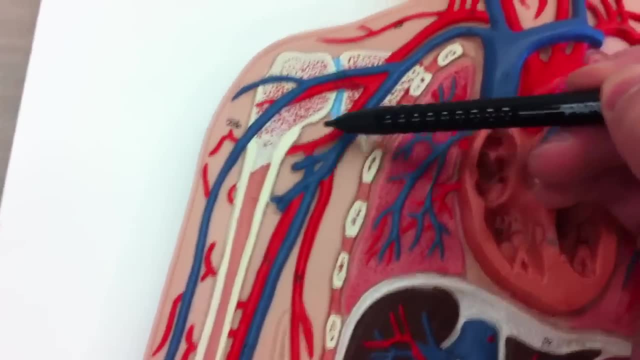 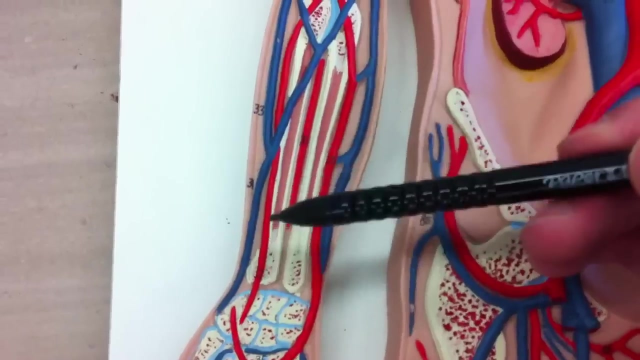 The left subclavian and the left common carotid each have their own direct connections to the aorta. If you follow the subclavian down, you'll have the axillary, which will be right here, And then the brachial artery, which comes down and splits off to the radial and the ulnar arteries. 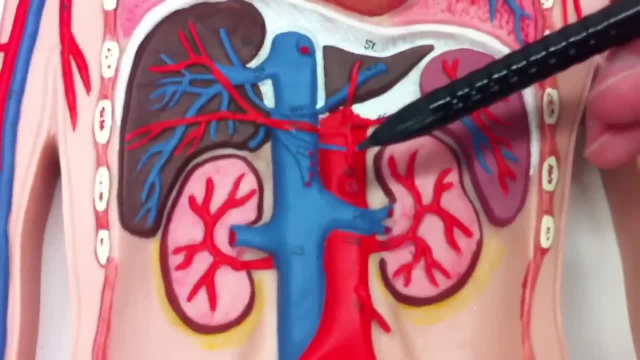 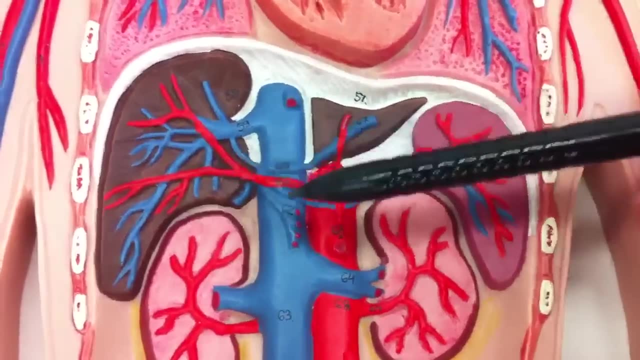 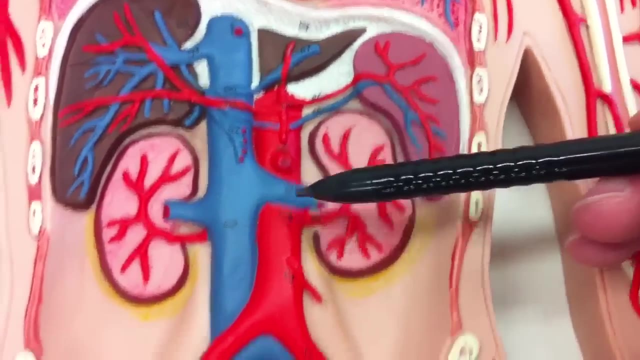 Coming back down to the inferior or descending aorta, we have the celiac trunk, which will have connections to the hepatic artery, and then the splenic artery. Right below that we have the superior muscle. We have the superior mesenteric artery and the inferior mesenteric artery. 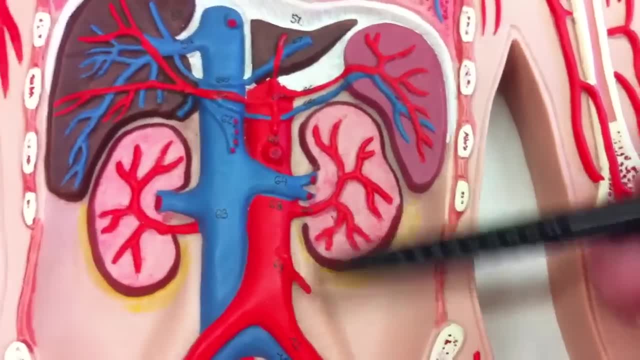 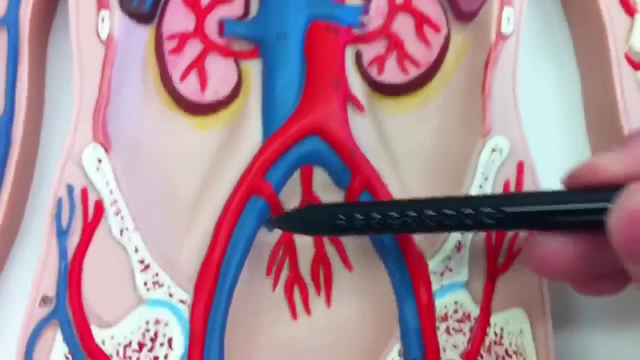 Between them you'll have- they're not shown, but the gonadal arteries too. And then you have the renal arteries. here that serve the kidneys, You have the common iliac iliacs- interior iliac- and the exterior iliacs which comes down. 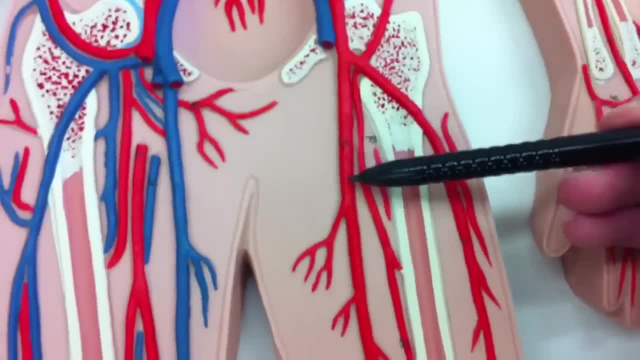 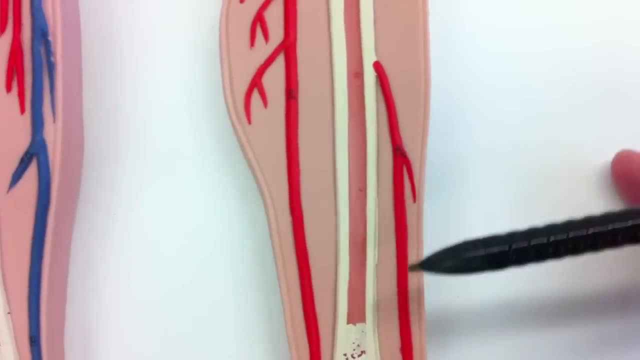 And you can't see it, but it's cut off. So the femoral artery will come down this way down. This will be the popliteal right here And then the The anterior tibialis artery and the posterior tibialis. 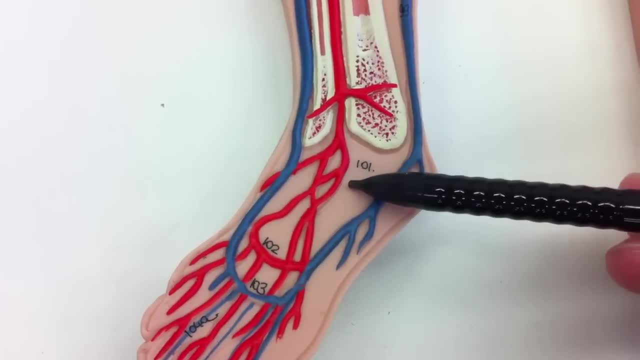 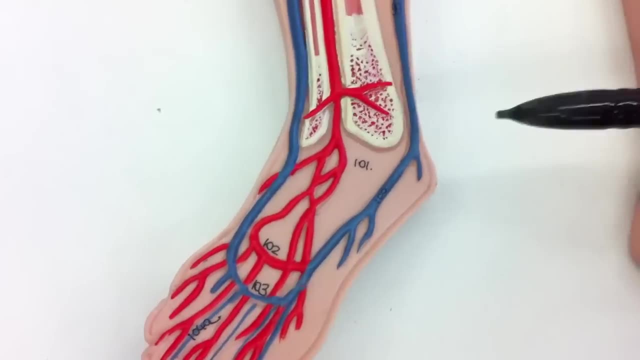 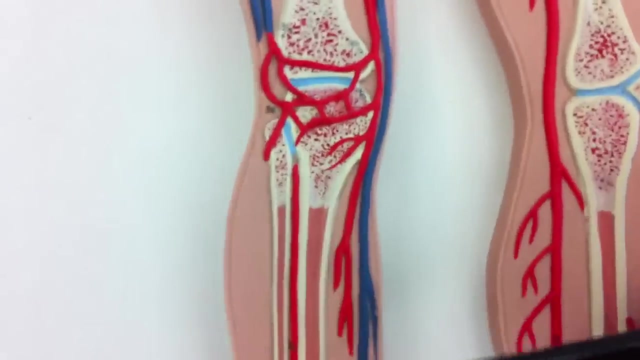 Down here we have the dorsalis pedis artery and then the arcuate artery down here. So that does it for the arteries, not for the veins. We have the arcuate vein right here and the dorsalis pedis vein. We have this really long saphenous vein right here. 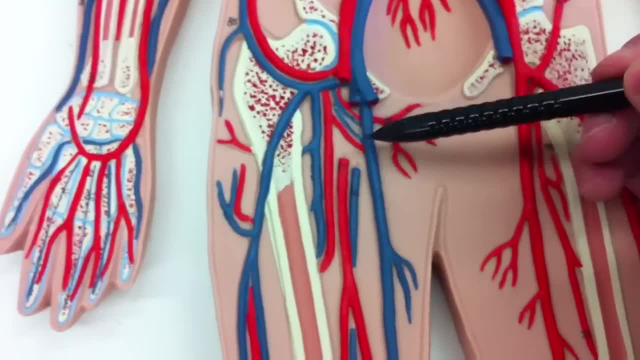 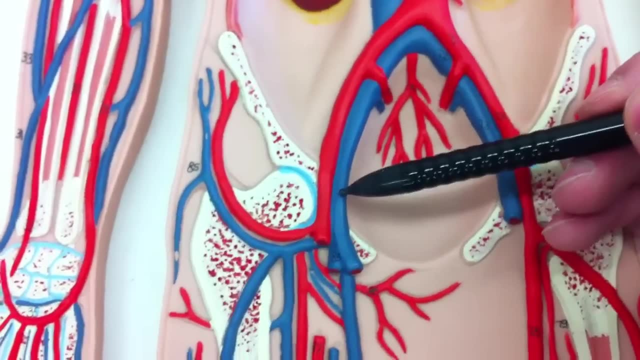 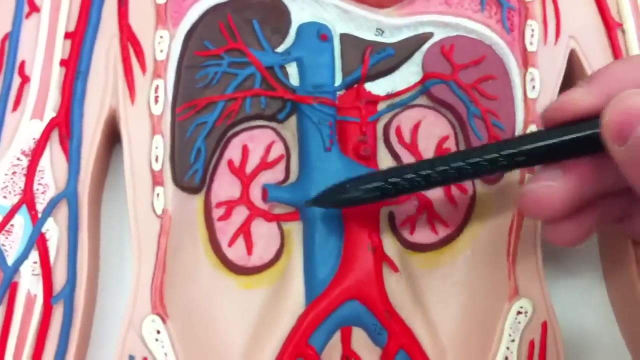 And then this one doesn't have it, but the femoral vein is cut off right here, but it should go down the middle. Then you have the common, or sorry, external iliac, internal iliac, common iliacs, And then the inferior vena cava. is this big guy right here? 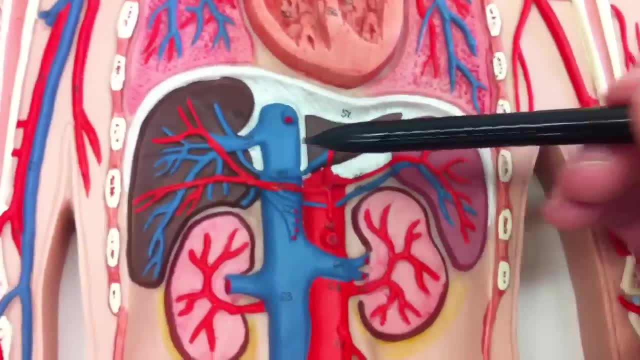 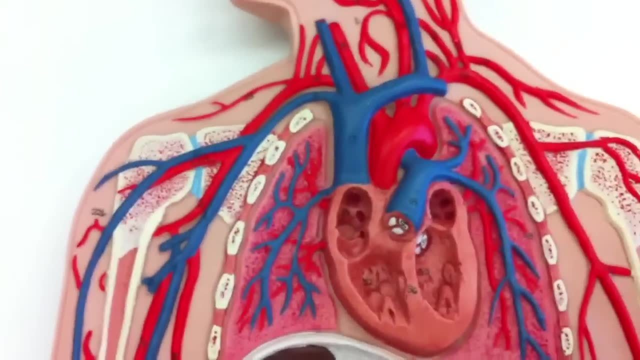 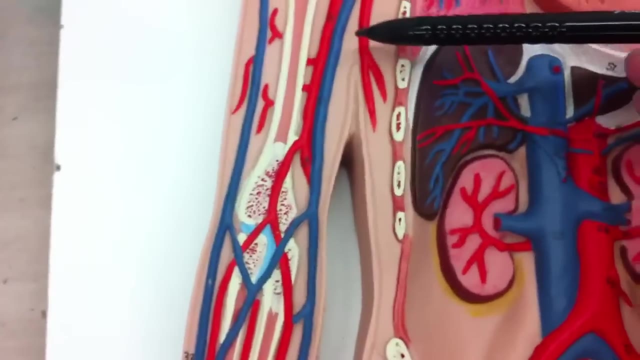 So you can see the renal veins right here, hepatic veins right here. There's a gastric and a splenic over here, And then over to the arms we have the cephalic vein, which is on the outside here, And then the 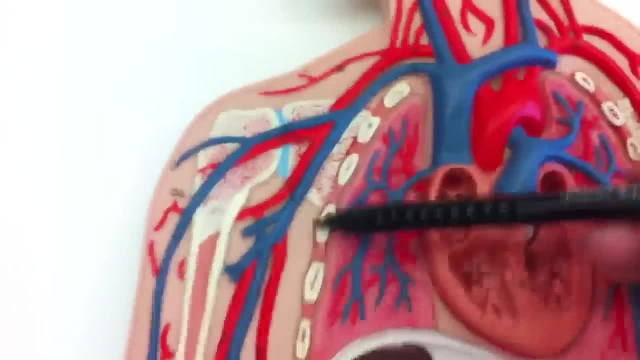 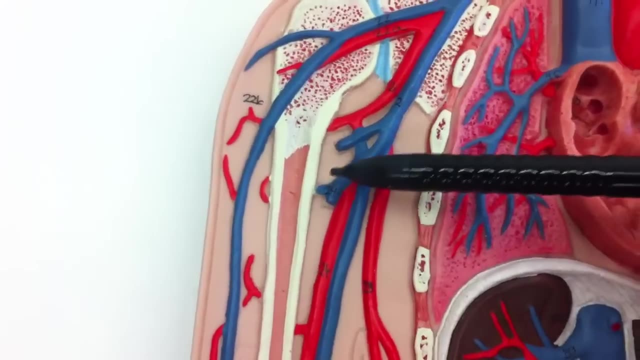